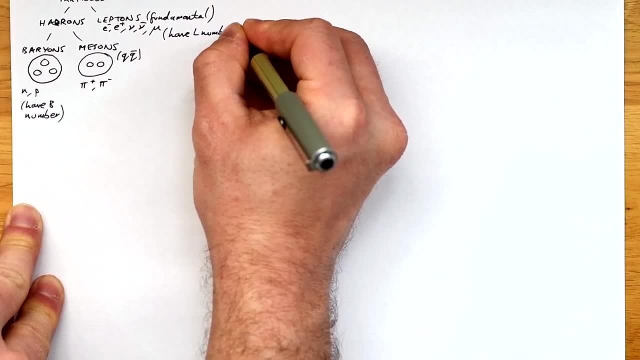 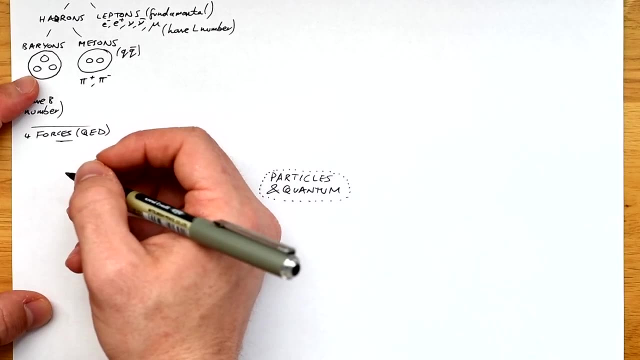 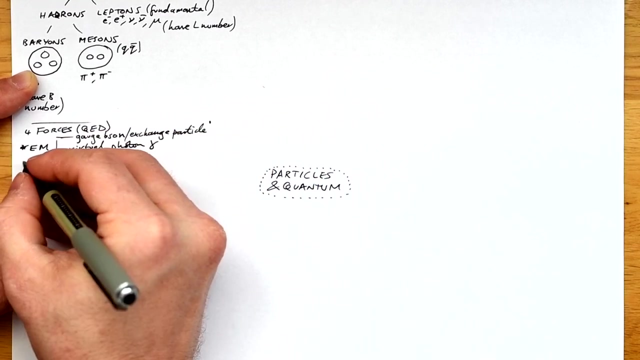 baryons have a baryon number and leptons have a lepton number. So let's talk about the four forces that we're concerned with in physics, Specifically in the area of quantum electrodynamics: the electromagnetic force, the gauge boson or the exchange particle, for that is the virtual photon, Strong nuclear force. 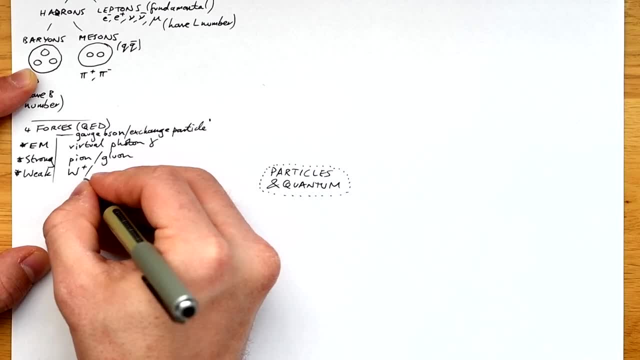 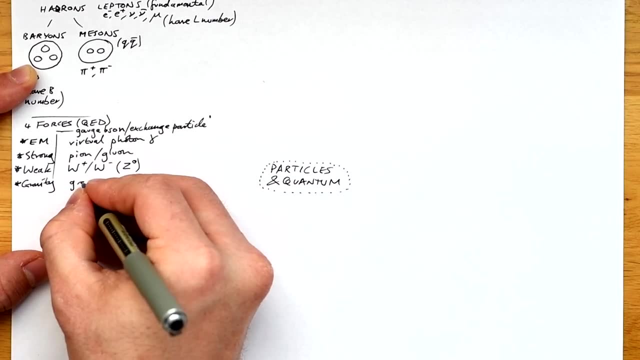 the gauge boson is the pion. sometimes you'll see the gluon Weak is W plus or W minus. we don't really deal with the Z zero And the cousin that we all ignore is gravity, because we don't really understand it as well And even though we haven't found it. 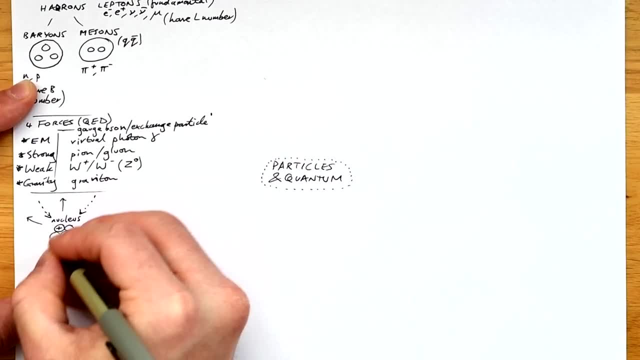 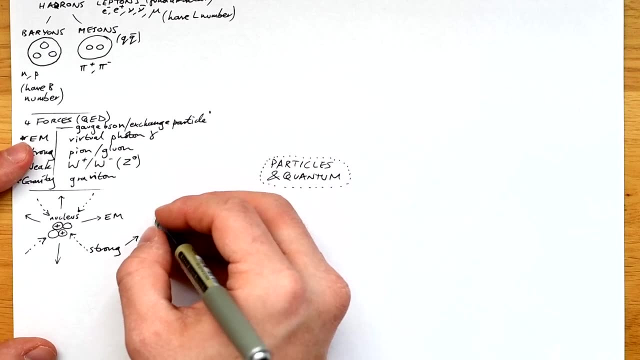 we call the exchange particle, the graviton. Okay, let's talk about the strong nuclear force, which is the force that's in the nucleus together. Of course, the electrostatic repulsion of the protons in the nucleus means that the EM force is always trying to explode a nucleus. So that means that we must have another force keeping it together, And that's the strong nuclear force, And that affects neutrons and protons. What's stopping the strong nuclear force from imploding a nucleus, then? Well, what we say is: when the nucleons get too close together to 0.5 femtometres. 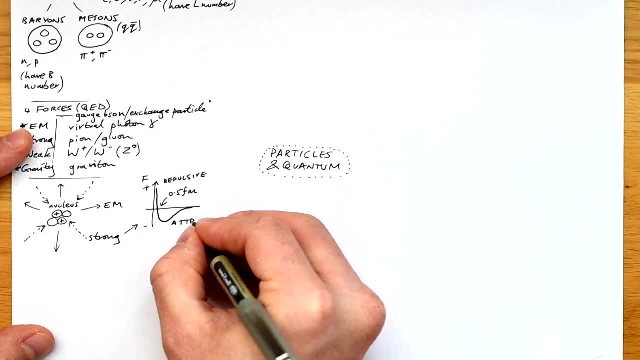 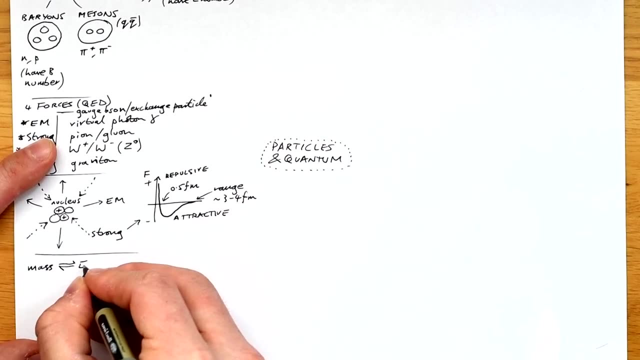 the strong nuclear force flips from being attractive to repulsive, And the range of attraction for the strong nuclear force is about three to four femtometres. Okay, so we know that mass and energy are interchangeable. The equation that links the two is the equation for rest energy. 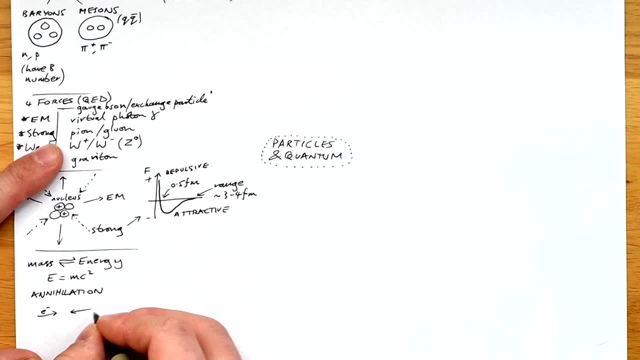 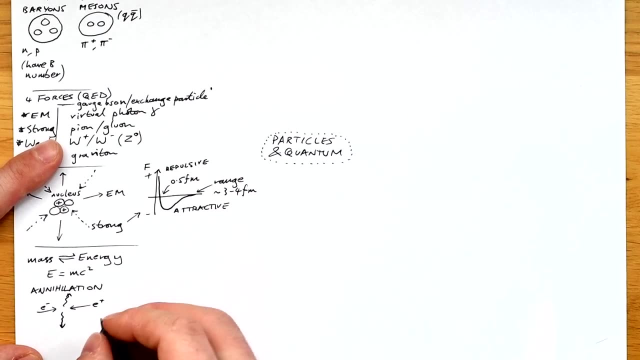 of a particle- and that's E equals mc squared Mass- is converted into energy in annihilation, That's when a particle and its corresponding antiparticle collide and they're destroyed and the rest energy is converted into photons. So we can say that E equals mc squared plus. 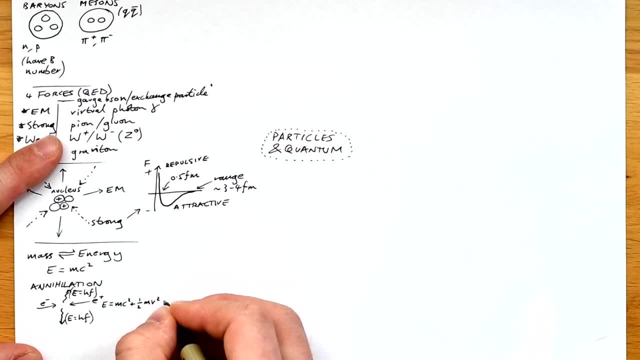 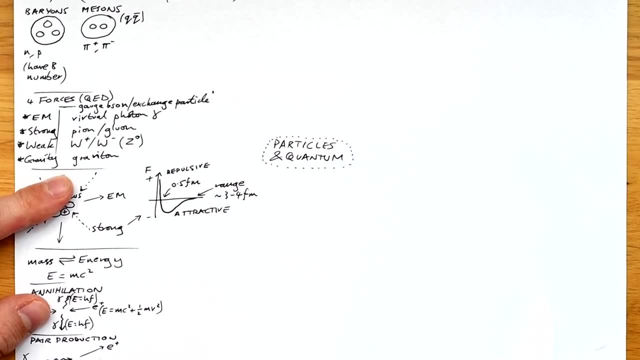 half mv squared. that's the kinetic energy of the particles going in with lots of HF coming out. The opposite is pair production, that's when a photon turns into two particles, Again a particle and its corresponding antiparticle, Of course. 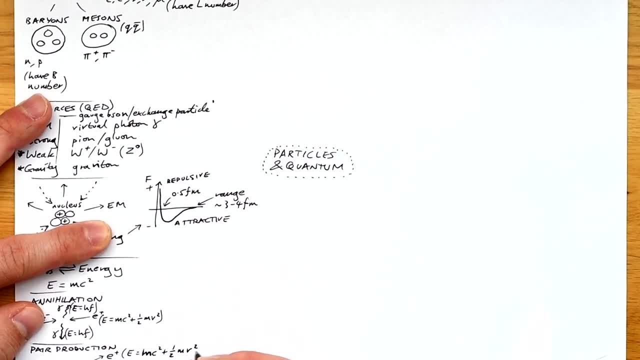 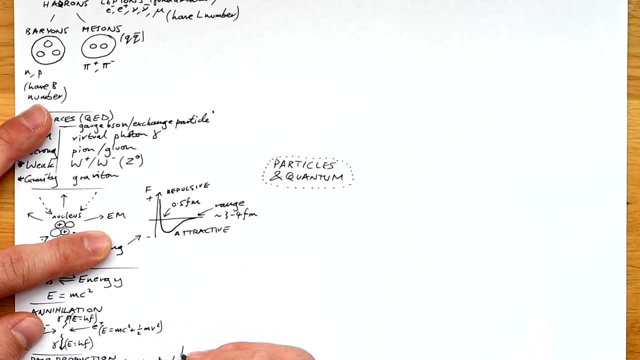 the photon must have at least the same amount of energy as the rest energy of the particles. So again, E equals mc squared. But if the photon has more than the minimum amount of energy, then the leftover energy is turned into kinetic energy of the particles afterwards. 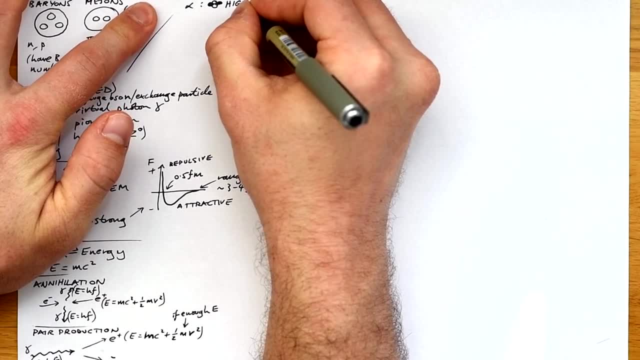 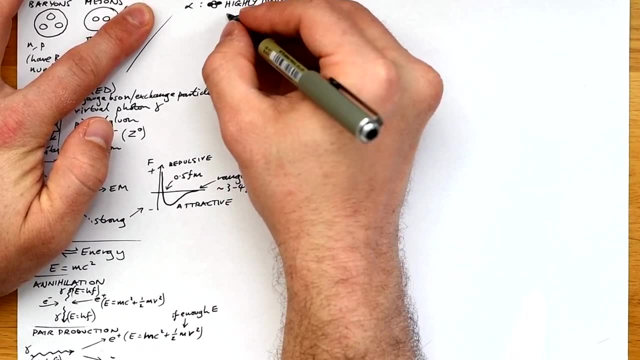 Okay, let's talk about ionising radiation: alpha, beta, gamma. I call them ionising radiation because all of these can give electrons Enough energy to escape an atom or molecule, therefore ionising them. An alpha particle is a helium nucleus, two protons and two neutrons. It's highly ionising. 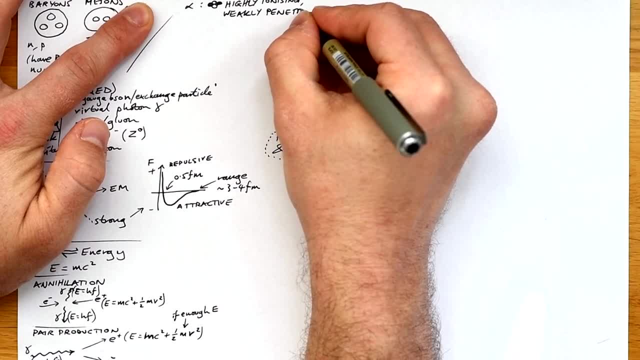 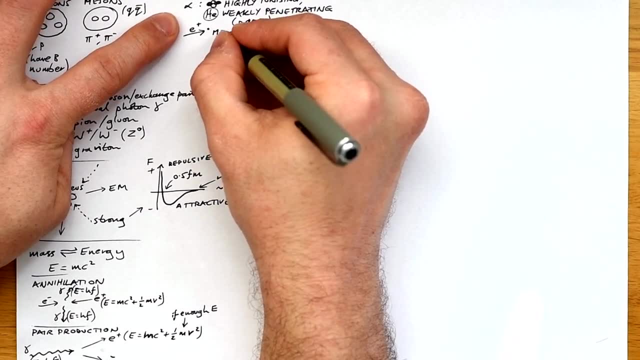 mostly because it's very heavy, but it's weakly penetrating. It's stopped by a piece of paper or a few centimetres of air. Beta particle is a fast-moving electron. Don't worry, I'll fix my mistake in a second. Then it has medium ionising and penetrating ability, stopped by a few. 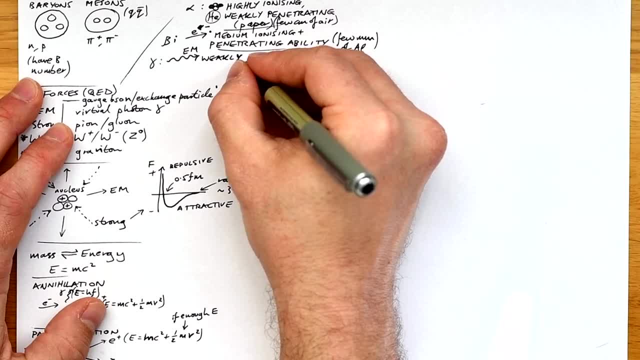 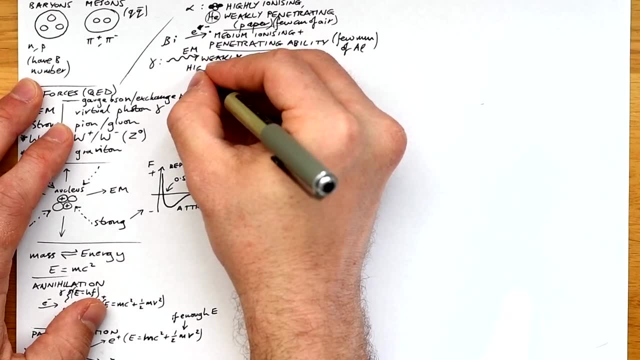 millimetres of aluminium. Gamma is just a high-energy EM ray or photon and that's emitted by an energetic nucleus. Photons don't have charge, so they can't change the nucleus in any way. when they're emitted It's weakly ionising but it's highly penetrative. It can't be stopped really. but 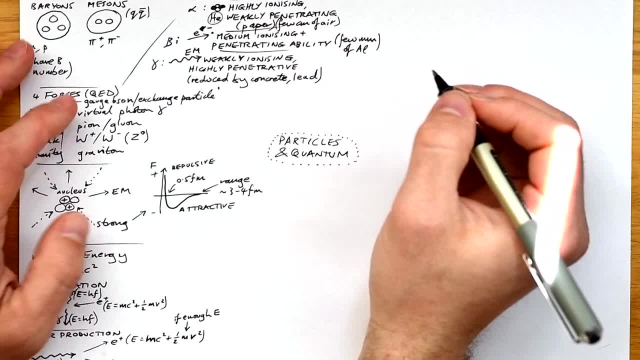 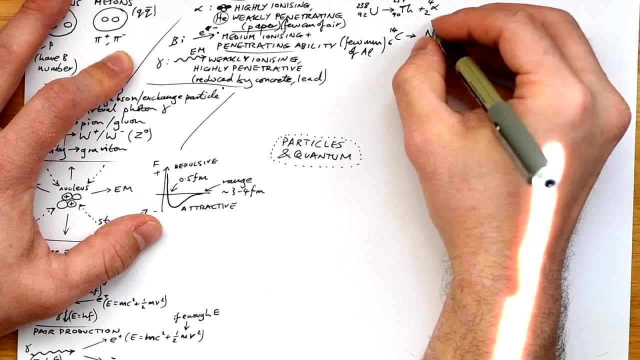 the intensity can be reduced by concrete and lead. Okay, here are the decay equations for alpha and beta. We know that alpha is four and two, beta is zero and minus one because it's got the opposite charge to a proton, and so therefore it's just. 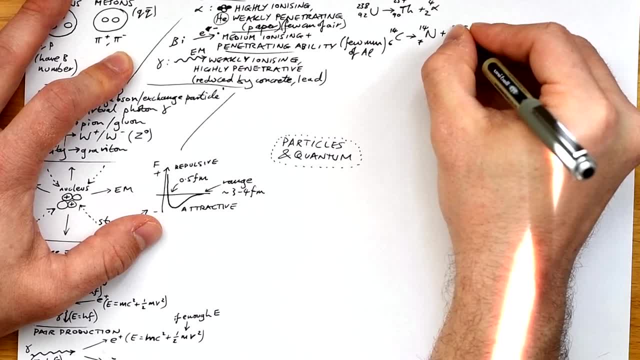 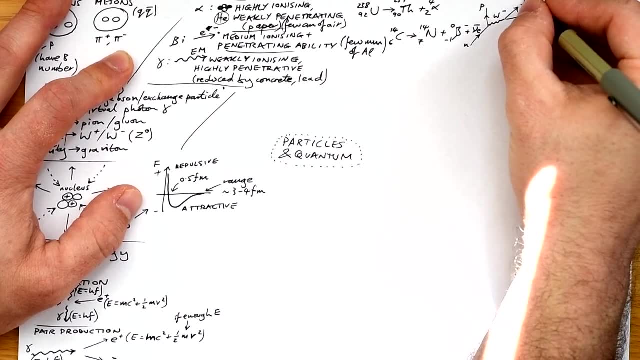 mass then, isn't it? Don't forget that for beta decay we must have an anti-electron neutrino produced as well, to make sure that lepton number is consistent Conserved. Here's a Feynman diagram for beta minus decay. We have a neutron turning into a 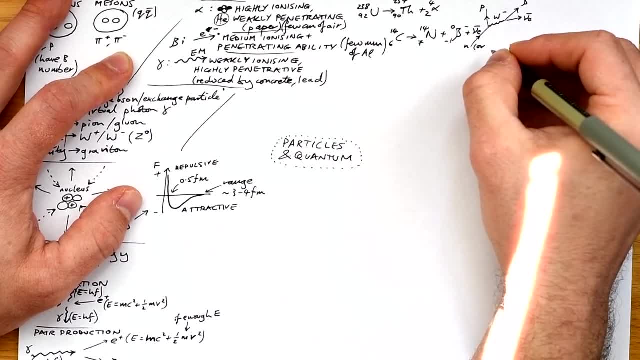 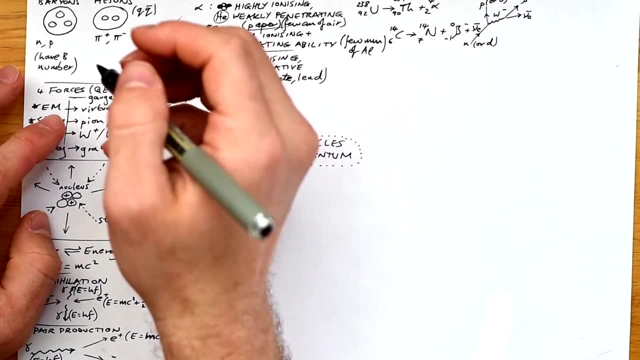 proton and the W minus boson takes the negative charge away, as it were, to produce an electron and an anti-electron neutrino. A neutron is up down down, Proton is up up down, so therefore we can say that actually it's a down quark turning into an up quark. You can see either one on a. 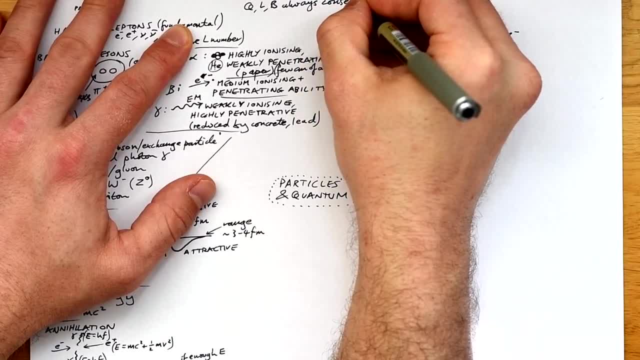 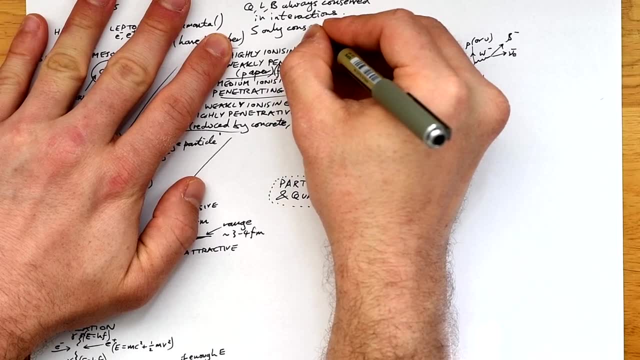 Feynman diagram for this. Okay, conservation rules. What has to be conserved? Charge lepton number and baryon number, Q, L and B. They're always conserved. Strangeness, however, is only conserved. 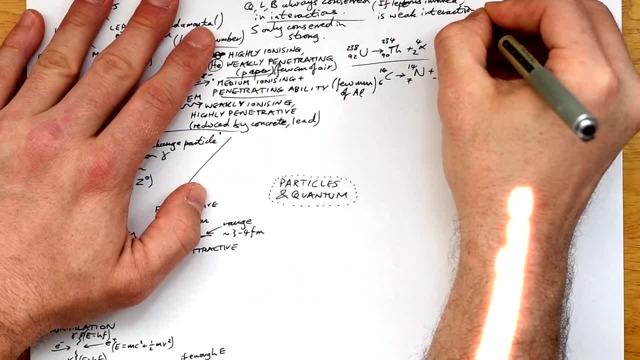 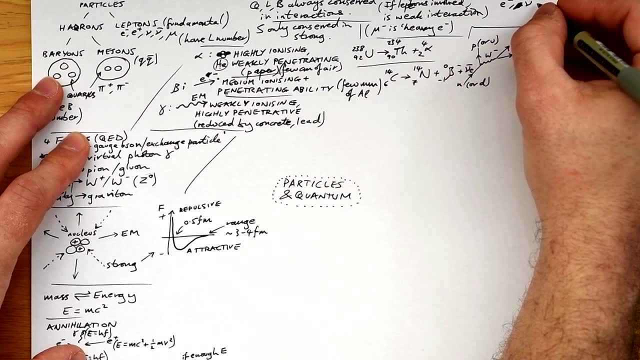 in strong interactions. Incidentally, any interaction that involves leptons has to be a weak interaction. It's good to be reminded about what a muon is- It's effectively a heavy electron- and a reminder that lepton number-wise electrons and neutrinos have a lepton number of 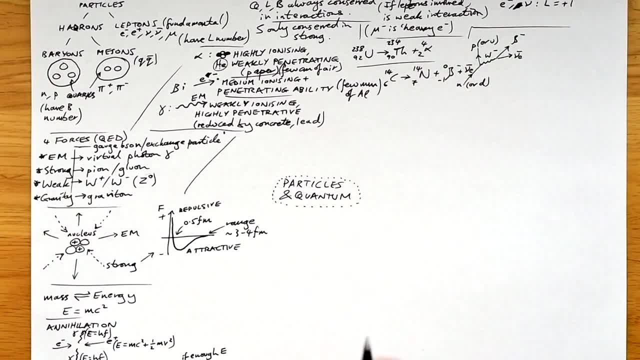 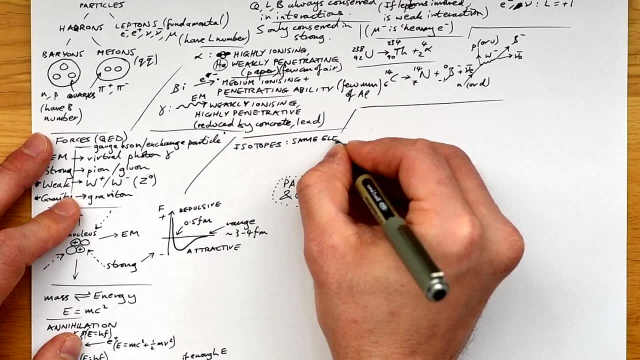 plus one, because the electron is the OG lepton, as it were. Positron has a lepton number of minus one. Okay, let's go back a little bit. Isotopes: what are they? Well, they're the same element. That means the same number of protons, or same atomic number. 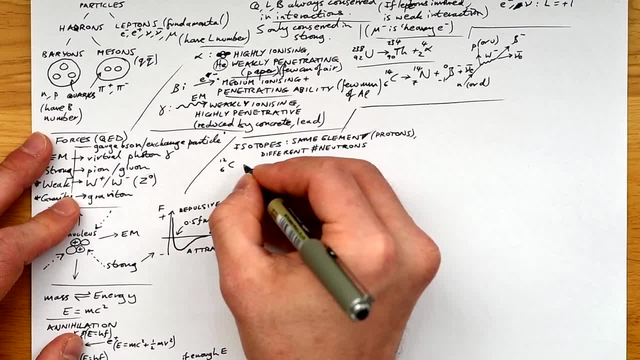 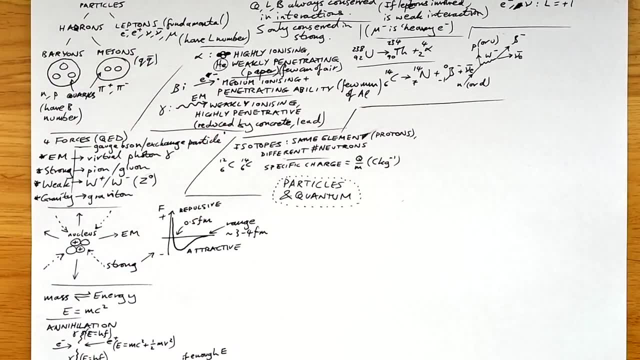 but with a different number of neutrons. so that means they have a different relative atomic mass, like carbon-12 and carbon-14. here Specific charge is the charge-to-mass ratio. so we calculate it by doing charge-to-volatile mass. so the unit is coulombs per kilogram, Generally a very big. 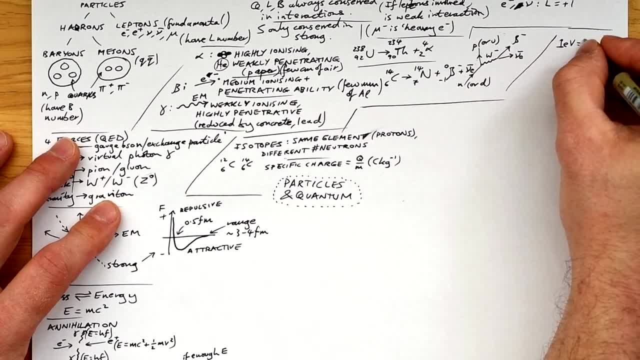 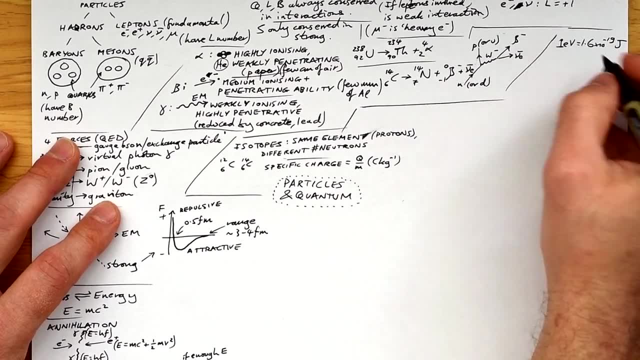 number because the masses of these particles are tiny, Worth remembering. the one electron volt is the same number as the charge of an electron, because one electron volt is the energy in joules that an electron has when accelerated through a PD of one volt. so that means that one electron 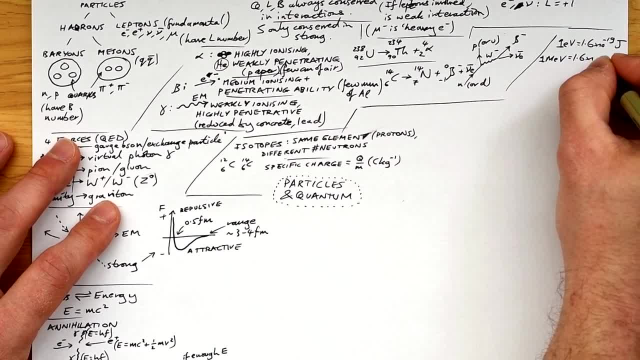 volt is 1.6 times 10 to the minus 19 joules. Quite often we deal with mega-electron volts and so if we have to convert that into joules, it's 1.6 times 10 to the minus 13.. Yes, you can. 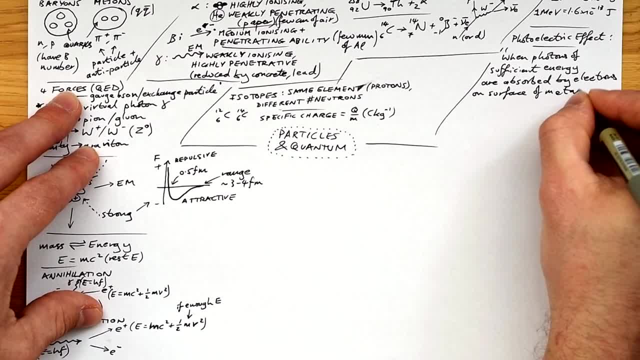 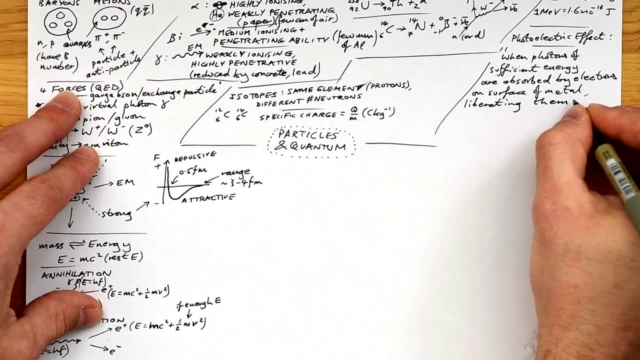 figure that out, but it's useful as a shortcut. Okay, so let's go on to some quantum then. What is the photoelectric effect? It's when photons of sufficient energy are absorbed by electrons on the surface of a metal. therefore liberating them, They escape. 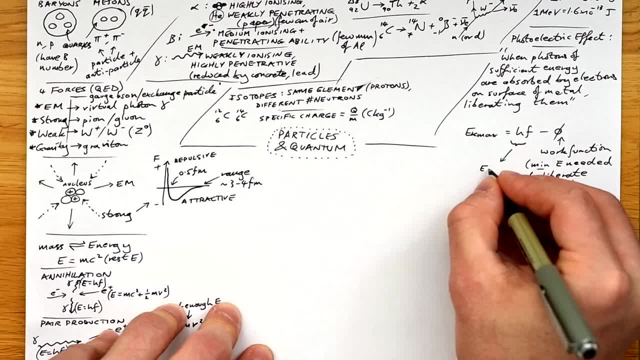 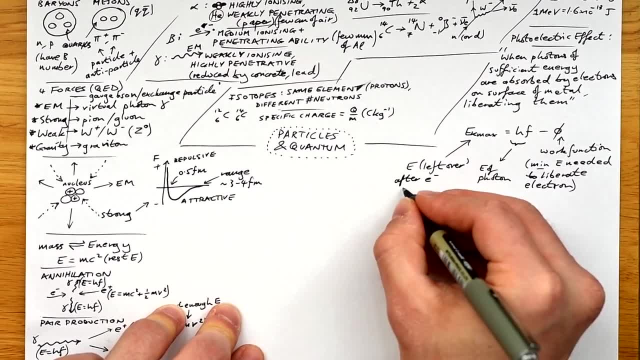 So we're going to use E. k max is equal to h f minus phi, H f being the energy of the photon that goes in, phi being the work function. That's the minimum energy needed to liberate electrons, and so taking one away from the other gives you the kinetic energy left when. 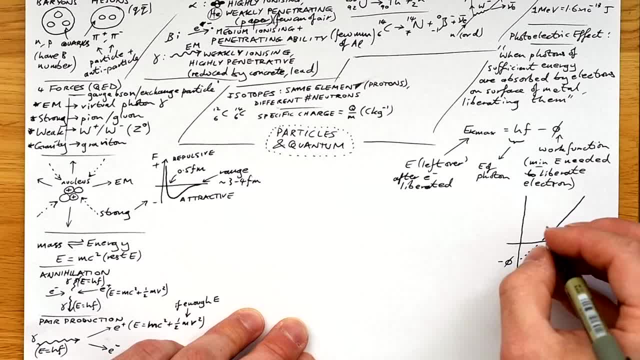 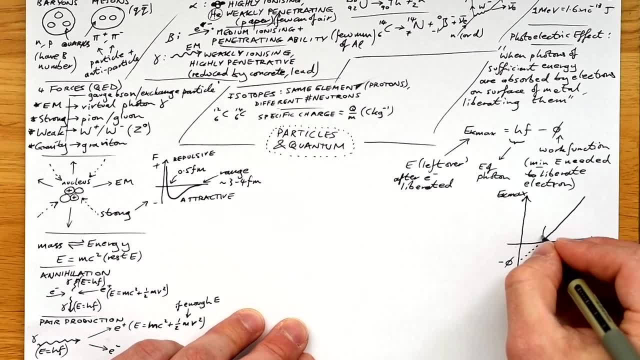 an electron has escaped. Here's the graph: The y-intercept is minus phi. The x-intercept is the threshold frequency. That's the minimum frequency needed for electrons to be liberated. If the frequency is less than that, you won't see any electrons liberated, and in that case 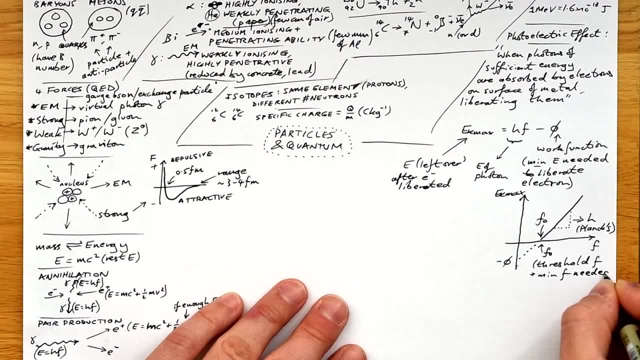 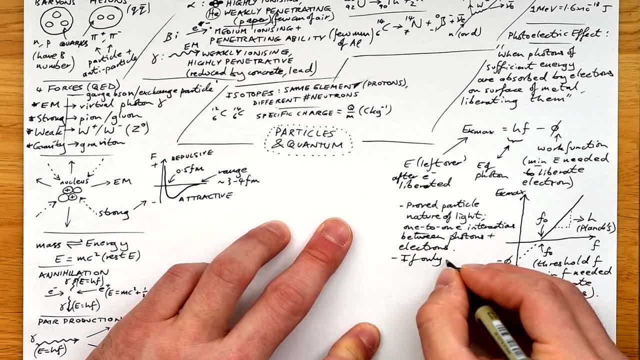 E k max is equal to zero. so h f zero equals phi. Okay, so what did the photoelectric effect prove? Well, it proved that light has a particle nature, not just wave nature, due to the one-to-one interactions between photons and electrons. 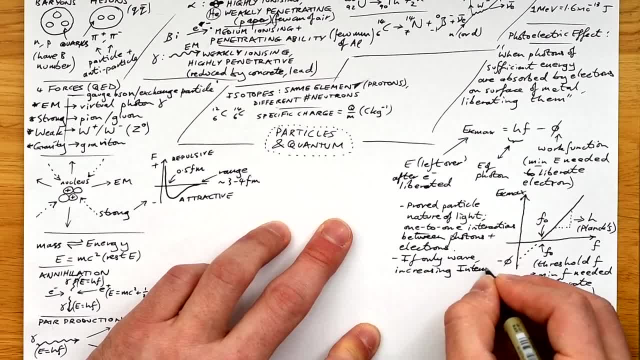 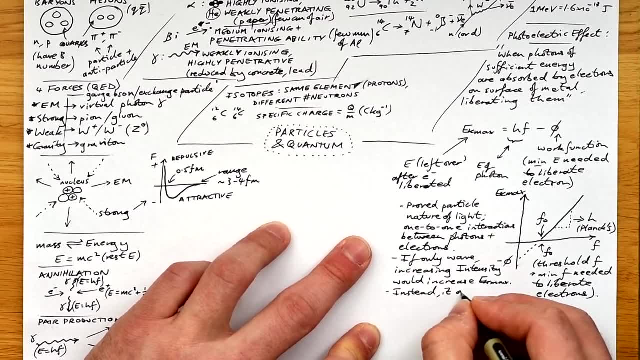 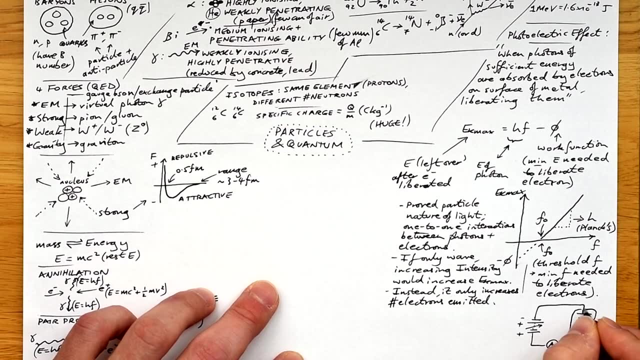 And it's one-to-one, because if it were only a wave, then increasing the intensity of light would have increased the E k of the electrons liberated. But it doesn't. All it does is increase the E k of the electrons liberated, So the light is not going to be separated. 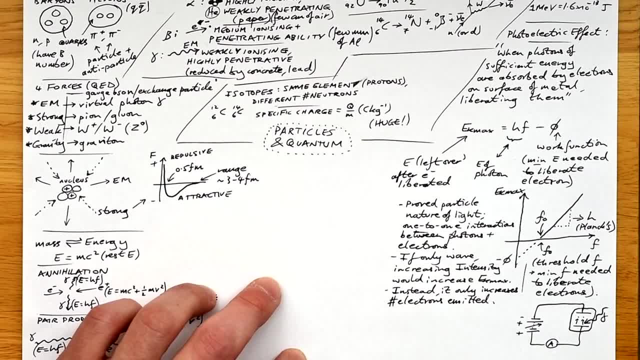 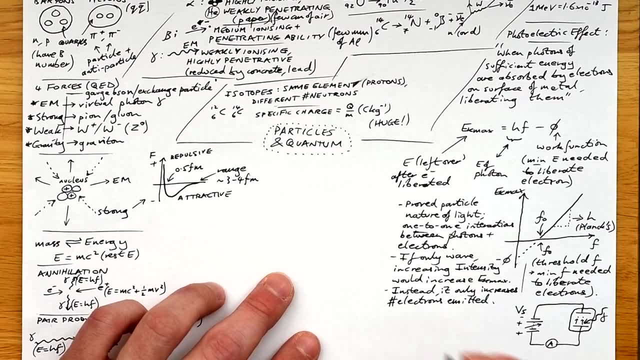 in the second because there are more photons. Okay, so here's a circuit that we can use to measure the kinetic energy of these electrons. We have a variable PD applied across these two plates. We shine light on one of them, specifically the anode, and that will make electrons cross the gap and then they will. 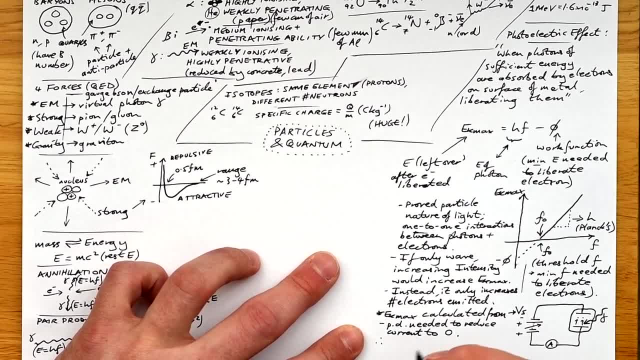 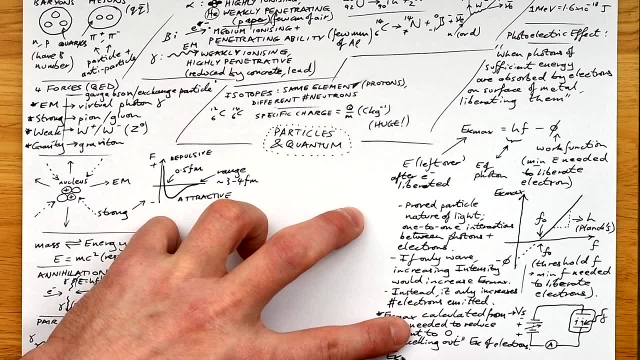 flow around the circuit producing a current. What we do is increase the PD in the opposite direction, as it were, until the current goes to zero. So the energy has been counteracted, as it were, by the energy supplied by the battery. 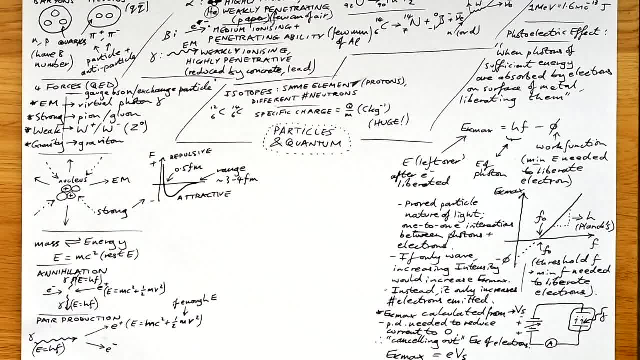 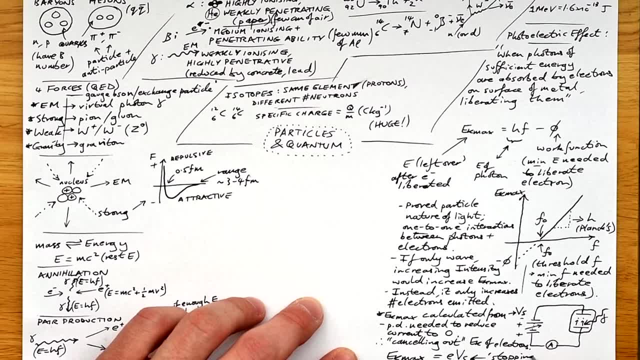 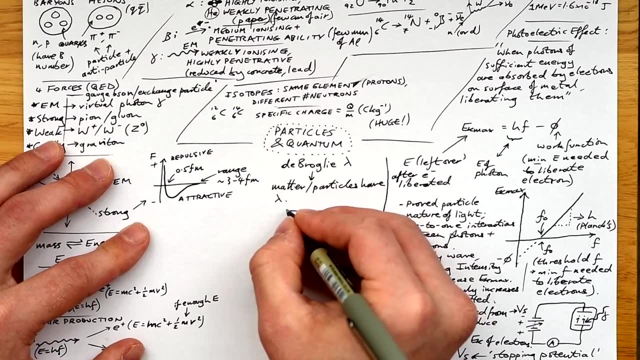 We call this PD the stopping potential And we know that any voltage is energy divided by charge And it's the same here. So we can say that E k max is equal to E charge of an electron times. the stopping potential for Vs A de Broglie wavelength is the wavelength 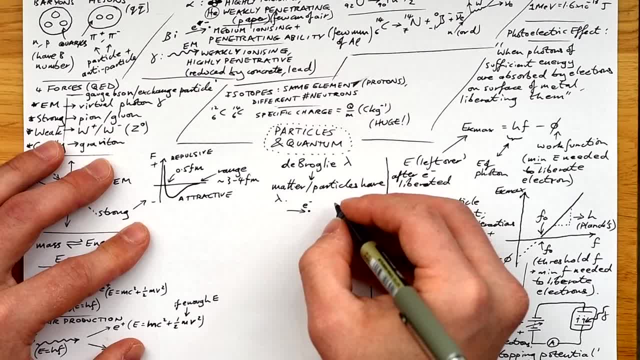 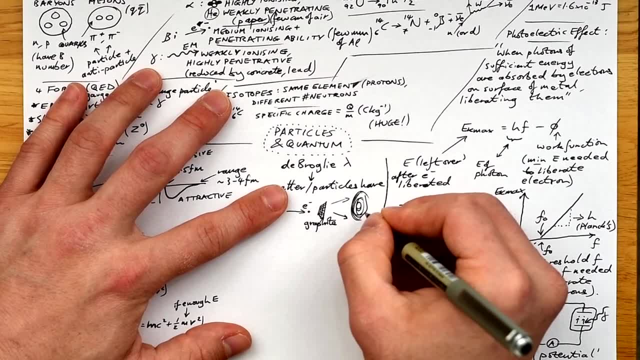 that a particle can have And the wave nature of particles was proven with electrons being fired at a ground level. So we have a graphite film and we see circular fringes on a phosphorescent screen behind, And that's because the electrons are diffracting around the carbon atoms and producing maxima. 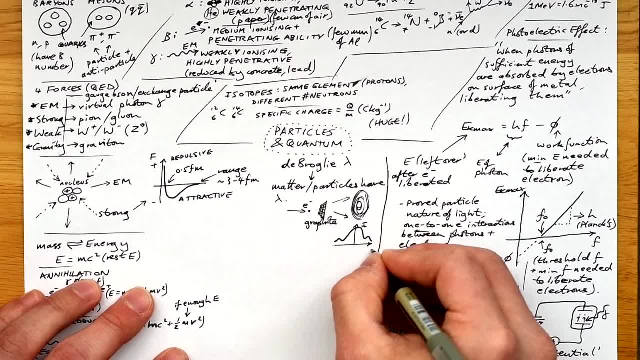 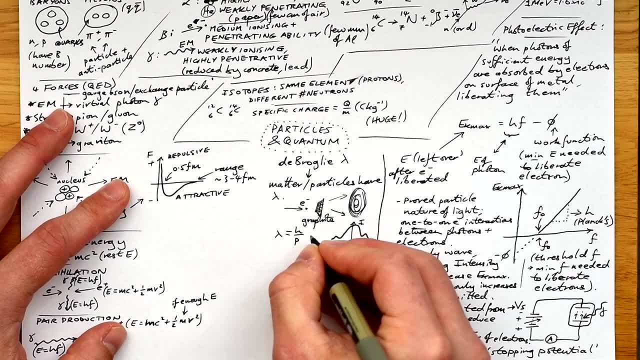 and minima on the screen, just like light. Here's the pattern for it. Note that the intensity doesn't really go to zero. De Broglie wavelength is equal to plex, constant over momentum, or h over p or h over mv. 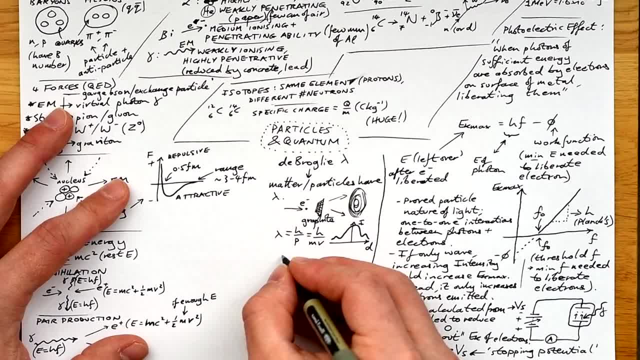 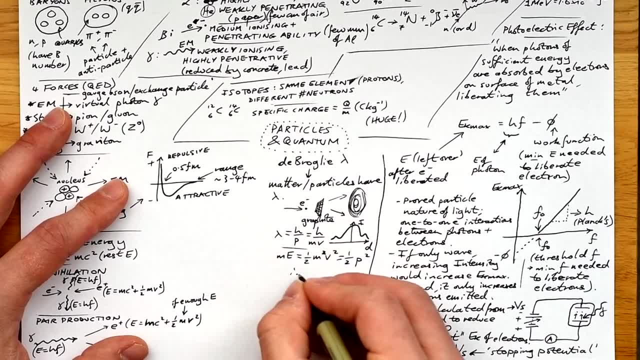 Quite often we'll be given the energy of electrons, but we'll have to find out the momentum in order to put it into the equation. So we find that by doing E, k, max, E equals half mv squared times the whole thing by m, and that gives you me equals half. 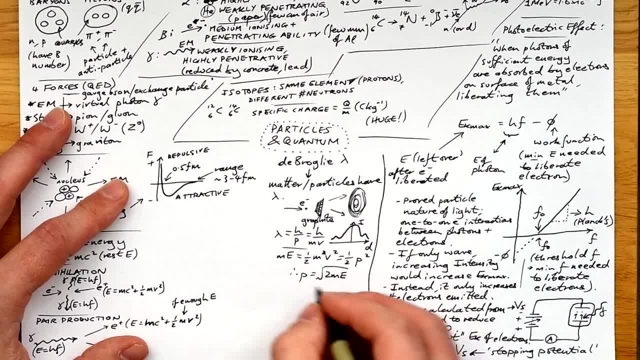 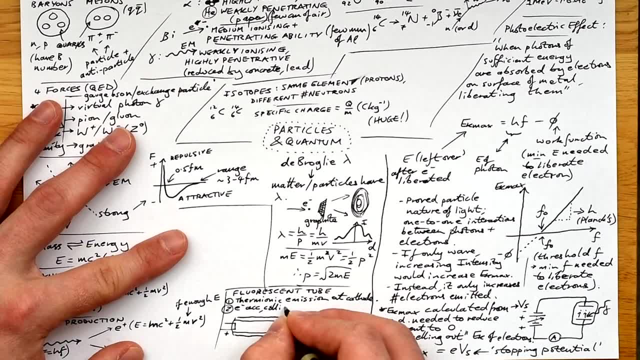 p squared Rearranging, we get momentum. p equals root, two m times the energy. Okay, fluorescent tube. What we have is a tube with a cathode on one end and an anode on the other end. The cathode is heated with a current, Electrons are emitted by thermionic emission. They're 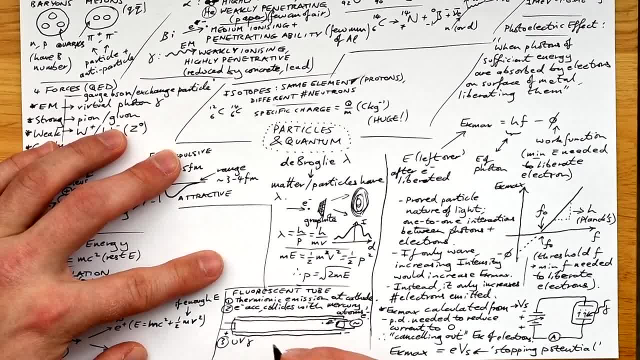 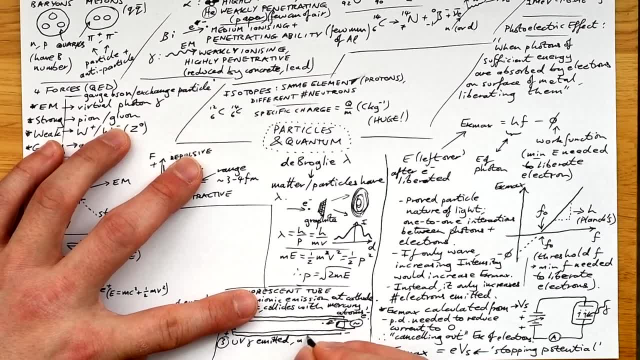 attracted to the anode on the other side and they bash into low pressure mercury gas atoms on the way. But what's the bigger thing? The battery, As you're building a nuclear plant, the batteryna быcositca are changing to the atom and that 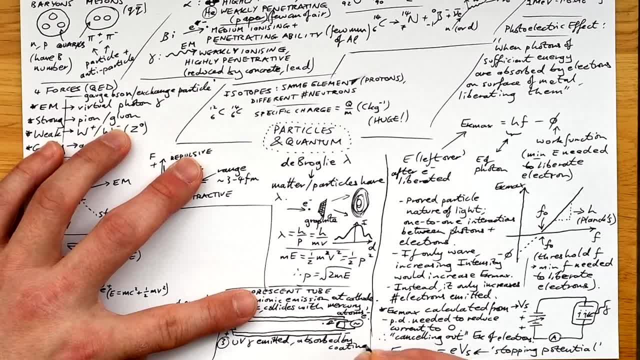 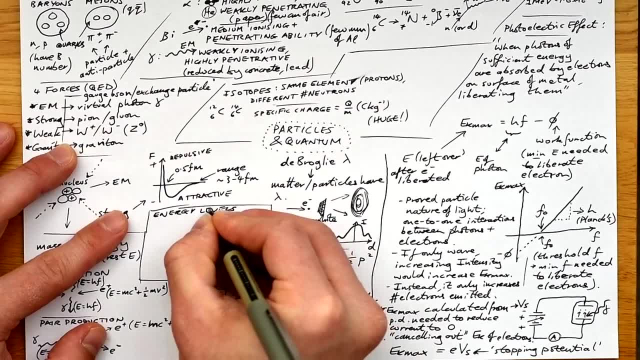 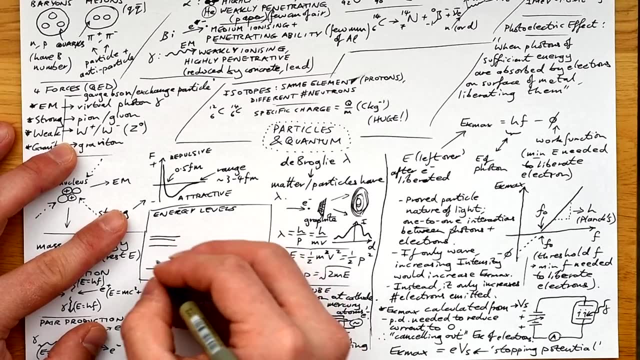 means they are attracted to the atomic atom first, before we can arrive at it on our planet. So we're saying: did you run off with this? Is this the time already? Do we have a chance? And maybe it is The fact all the time. if the process is measured at the same temperature, then Brother can.